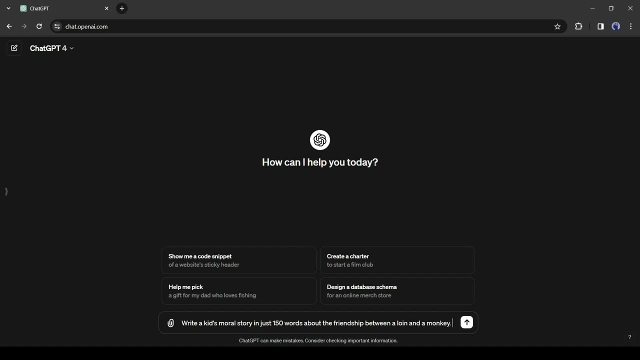 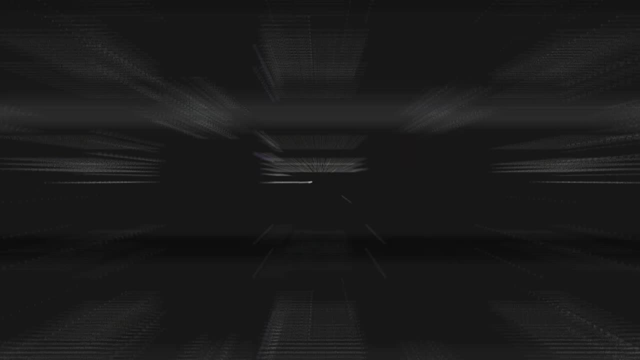 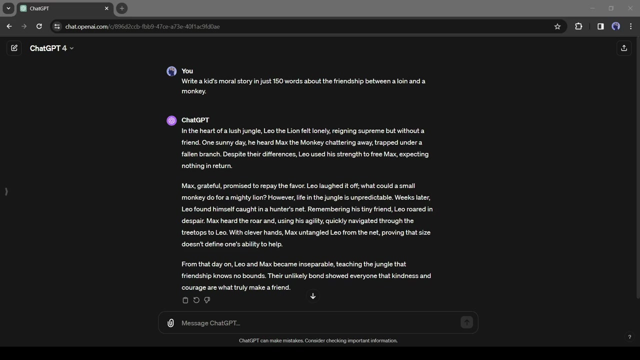 between a lion and a monkey. here I mention 50 words only for tutorial purposes. you can mention as per your wish. Then enter your story topic and hit the enter button. And here it is. Our story is ready. Now I will enter another prompt to generate image prompts. 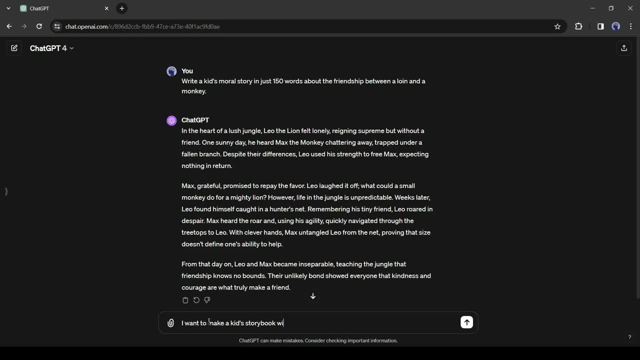 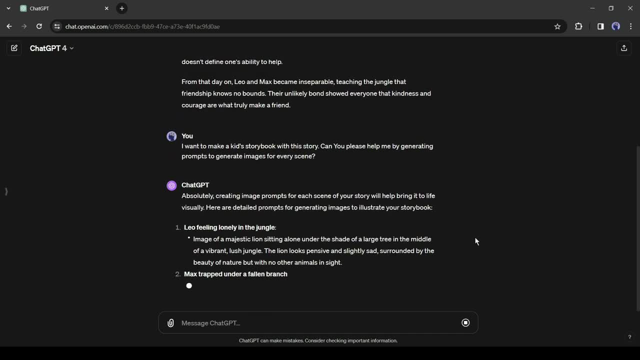 Simply type. I want to create a kid's storybook with this story. Can you please help me by generating prompts to generate images for every scene? ChatGPT generates image prompts for us And the prompts are really amazing. But there is a catch. 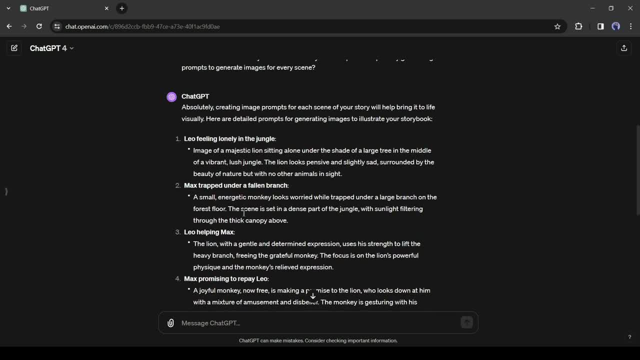 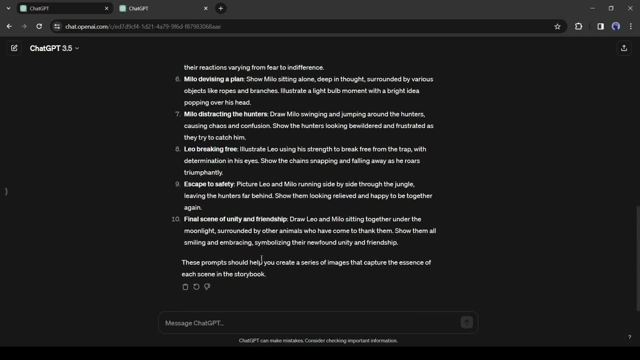 I generate the prompts with GPT-4, and it's paid. If you are using the free version, then your result might be like this one. It mentions the characters main in prompts, but there is no character description. To solve this issue, Just enter another prompt. Please add their. 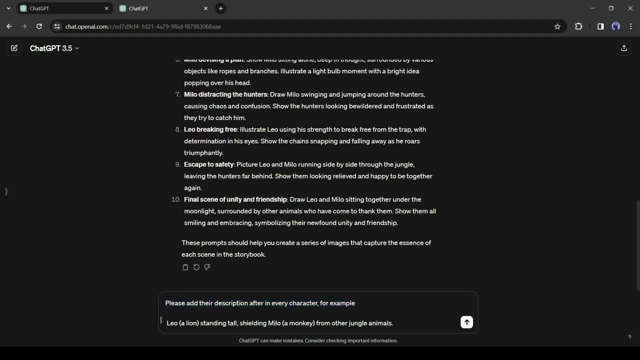 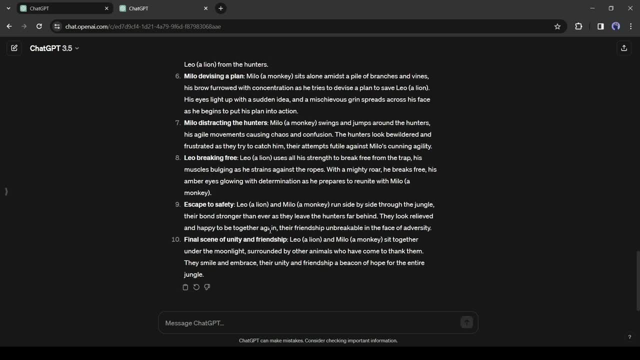 description after every character. After that, enter an example like me and hit the enter button. And now our image is created and υFl cute. I will give you an example. To begin, I will press reasonies. image prompt is ready. Now let's move forward to the next step After generating the story. 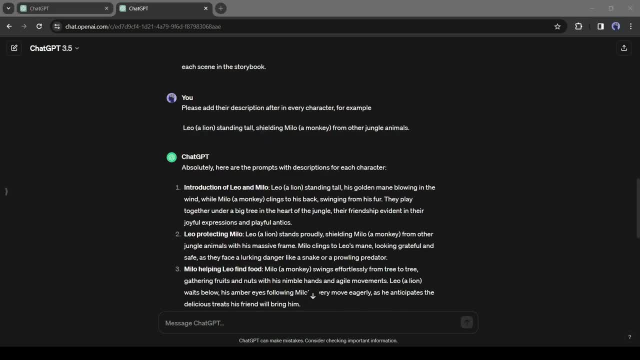 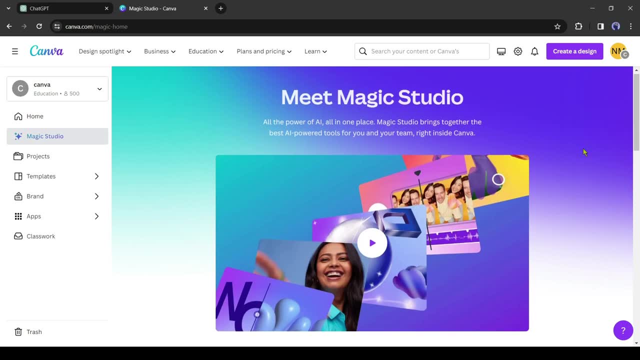 now it's time to generate the image and book layout, And to do this, I will use Canva. Canva is a well-known tool for designers. Now it's become more powerful with various AI tools. Alongside their own AI feature like Magic Media, you can use a vast number of third-party popular 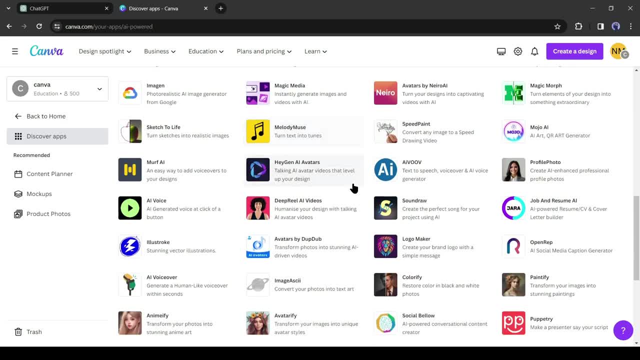 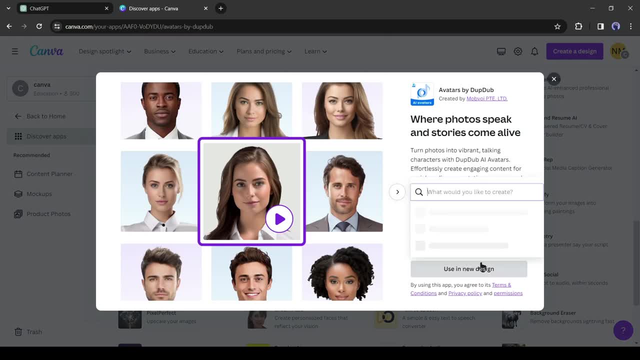 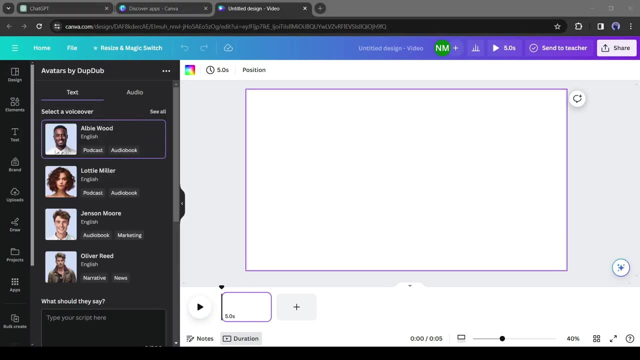 AI tools like Dulley Muff, Hagen, DubDub and many more. For example, if you want to use Avatar by DubDub, select the tool. After that, create a new design or use an existing design. After creating the design, your interface will be like this one. There are two options to create an. 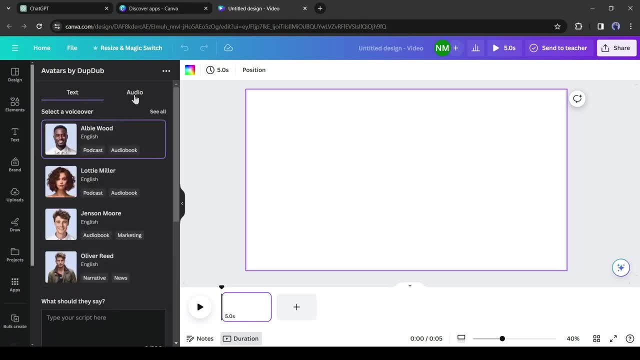 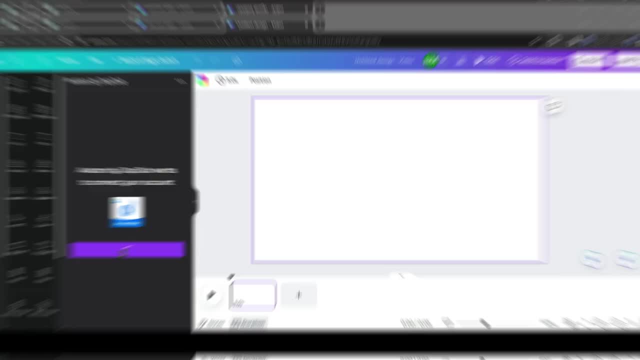 avatar. You can generate a voiceover with DubDub or upload your existing audio clip. First of all, click on sign in to DubDub from here and then log in or create a new account on DubDub After that. to generate a voiceover with DubDub, select a voice actor from here. Click on see all from here to find the voice actor. After that, to generate a voice over with DubDub, select a voice actor from here and then log in or create a voice over from here. First of all, click on see all from here to. 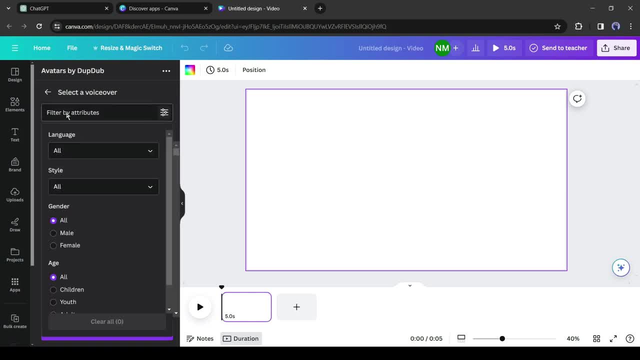 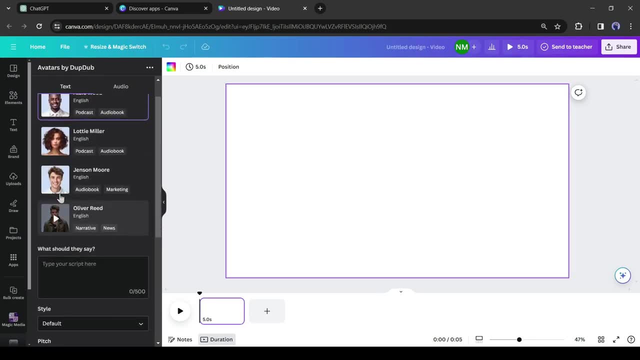 find all the voiceovers. You can use a filter to find the best one. Set your language, style, gender and age. After that, listen to some of them and select the best one. After selecting the voice actor, enter your script. Next, select a style or emotion. 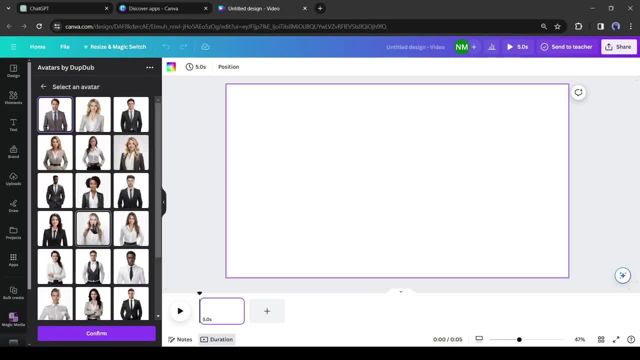 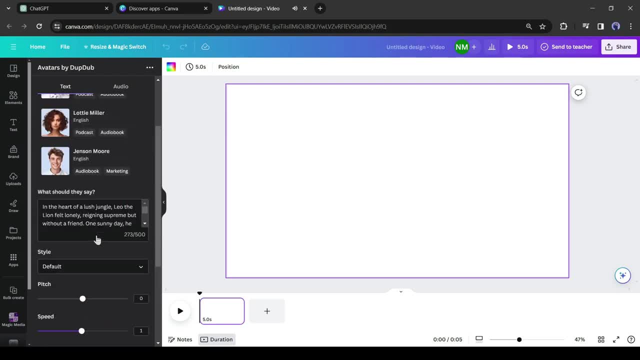 Then adjust pitch and speed And, in the end, select an avatar from here. After all is set, you can hear the preview of your audio. If you are satisfied, then click on generate talking photo from here. It will take some time. 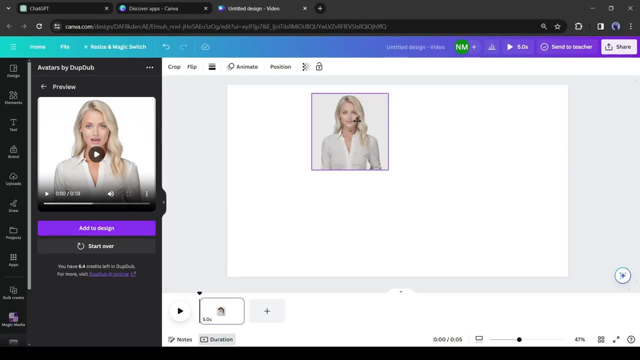 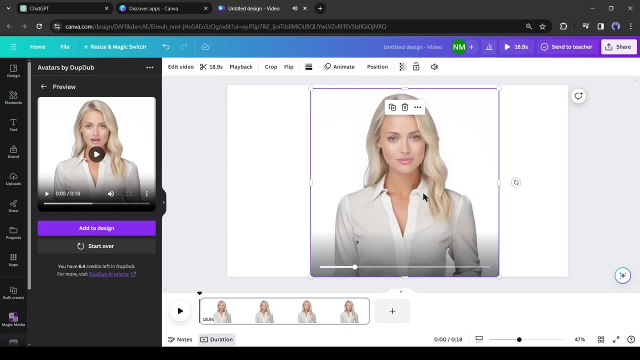 And here it is: our avatar video is ready. Now you can use it on your video. In the heart of a lush jungle, Leo the lion felt lonely, Reigning supreme, but without a friend. One sunny day He heard Max the monkey chattering away, Trapped under a fallen branch. 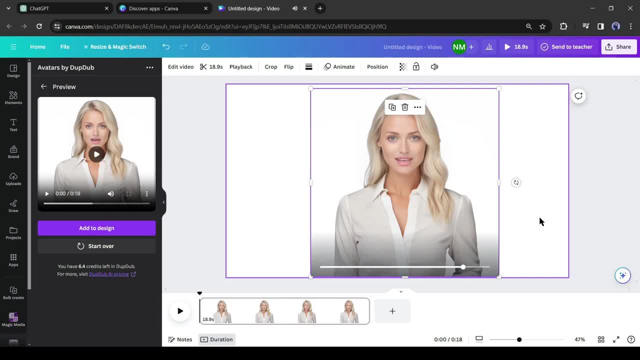 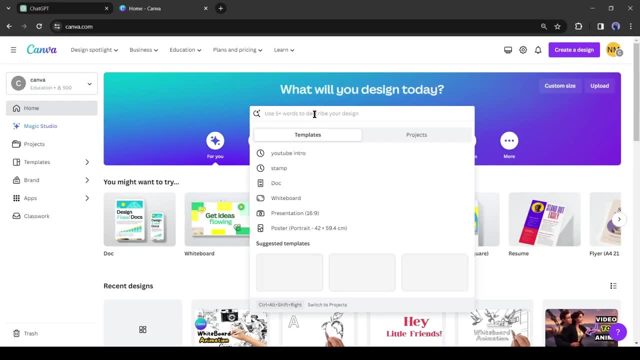 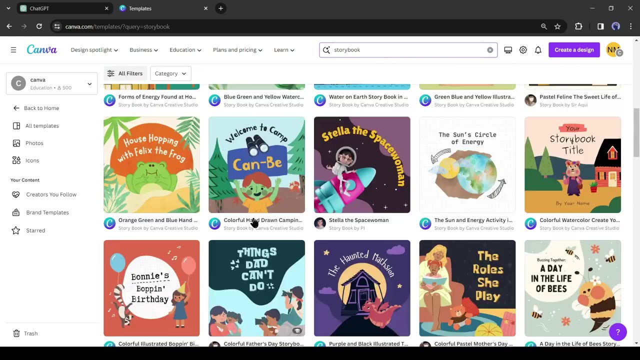 Despite their differences, Leo used his strength to free Max, Expecting nothing in return. Alright, let's move to the kid's storybook creation journey. Come to the Canva homepage and then search for the storybook in the search bar. You will find a vast number of storybook templates. I will suggest to start with blank. 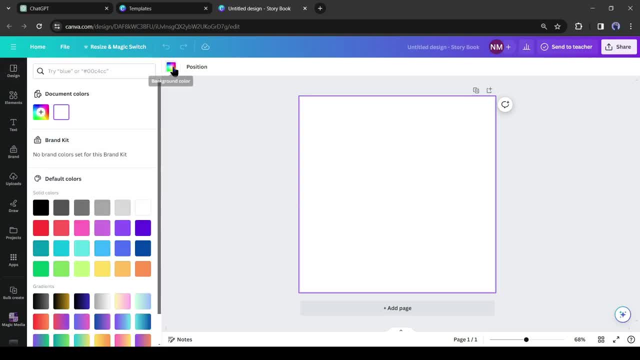 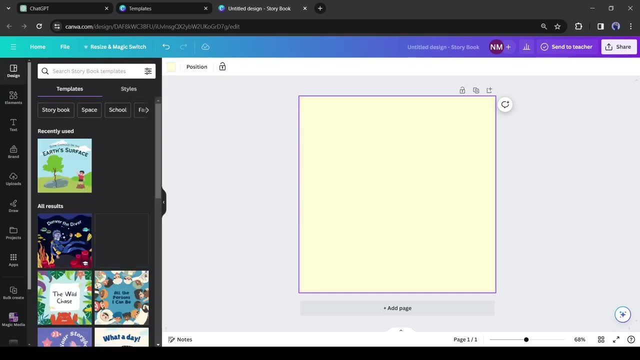 And this is our storybook creator page. first of all, change the background. let's leave the text blank. Now we want to add a frame to place pictures related to our story inside it. Go to the elements section, then open the frame section. 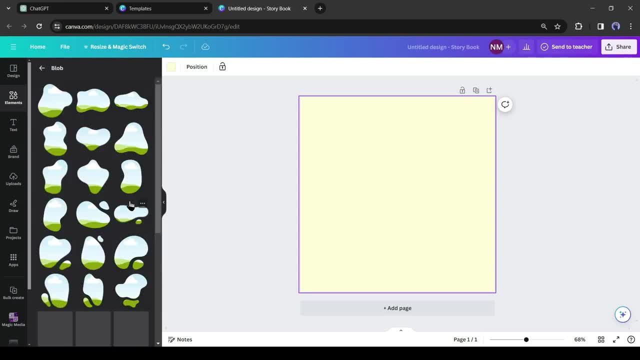 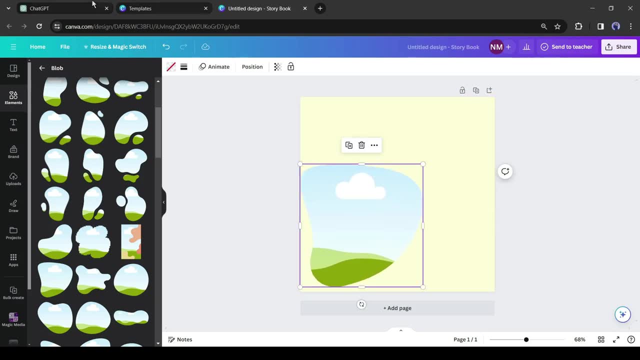 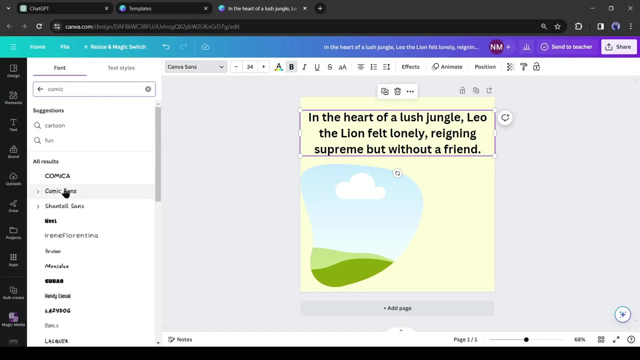 After that, open the blob section. I will use these shapes in my book to place the image inside. Now browse these many shapes, then add the one you like. next, Add the first section of a story as text on the first page. Now change the font type of the text to Comic Sans. 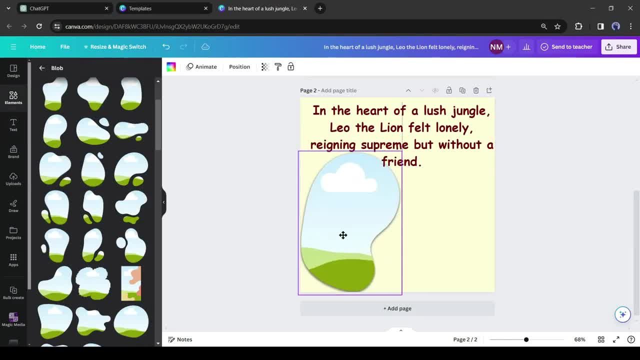 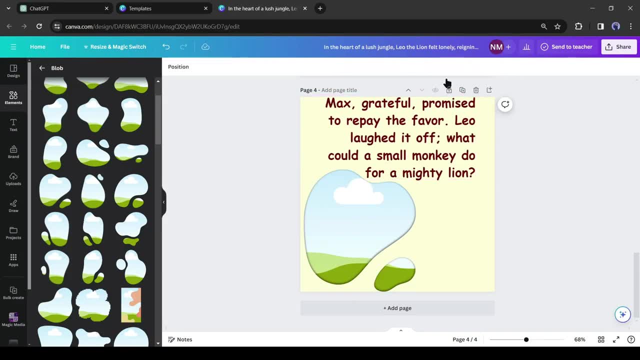 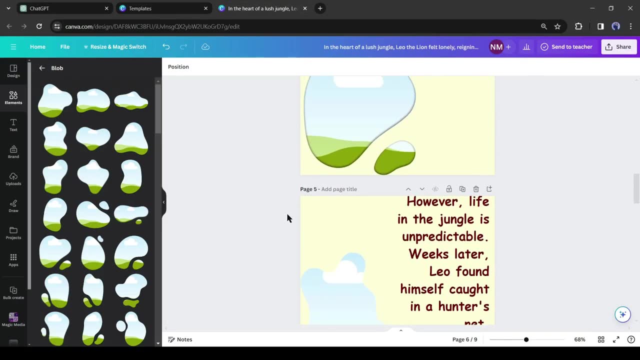 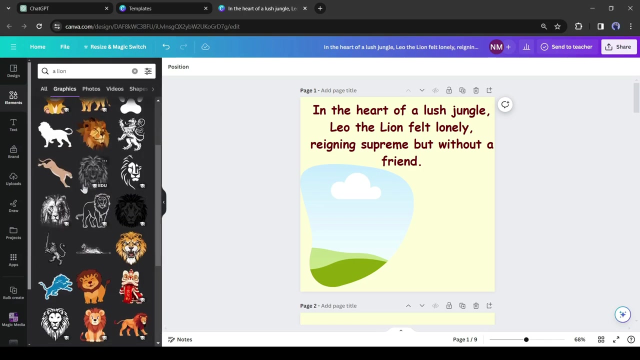 Sans. In this way I complete the creation of the rest of the pages of the story. Add storylines on each page in an appropriate manner. The next step is to add decoration to the pages. Open the elements section, then type a lion in the search box. We will add. 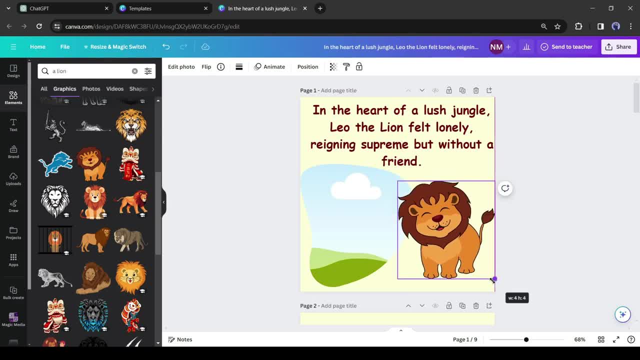 one of these cute pictures from the graphics section to the front page. After that, open the transparency and reduce the value to 40.. We want to make the image of this lion transparent behind the text, to give aesthetics to the page In this way. continue adding interesting. 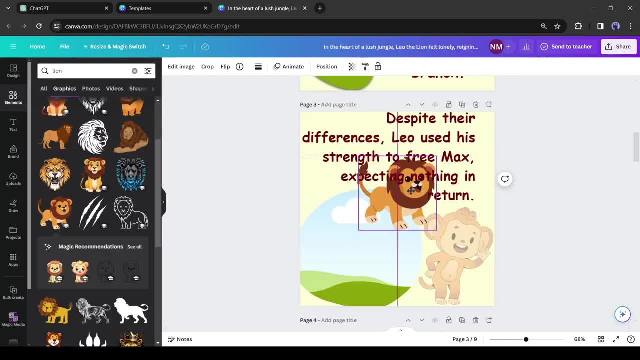 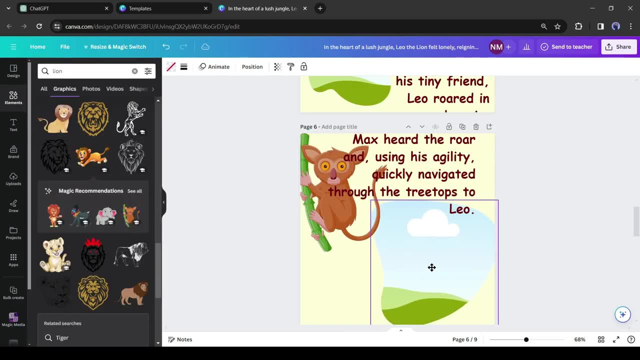 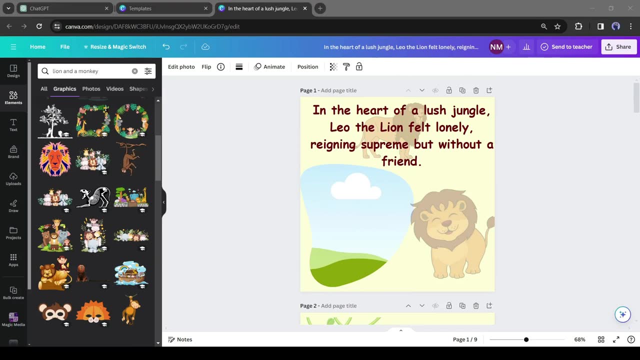 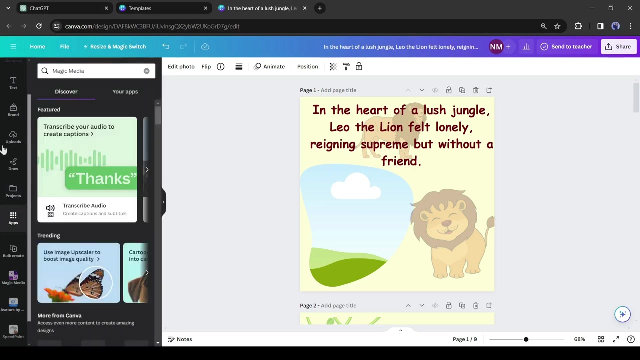 shapes and images to the rest of the pages, then make them semi-transparent. All right, our pages are ready. now we have to generate images with the prompts and insert them on the frame. We will now use canvas free image generator. Open the applications section on the left. Now search for magic media on the search bar. 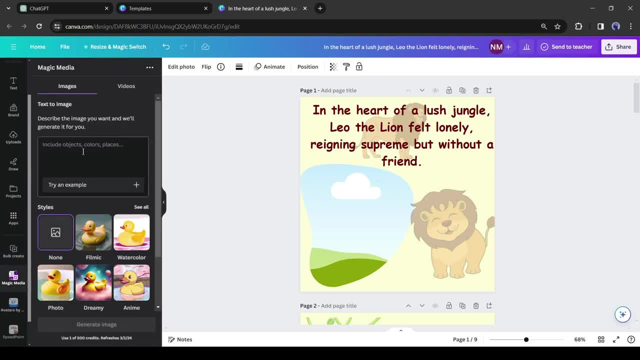 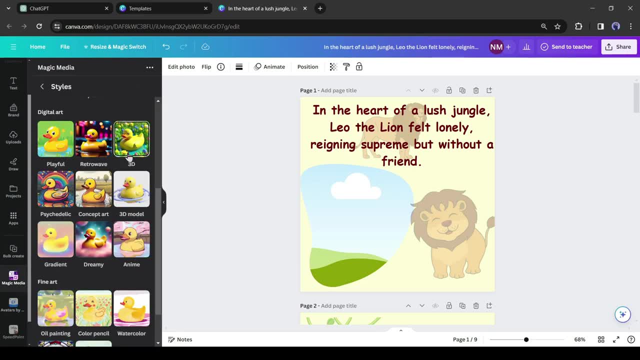 After getting the search result, select the magic media tool. Here you can generate images or videos from text prompts. First we have to select an art style. let's try with the 3D option. After selecting the art style, go back to chat GPT and copy the first image. 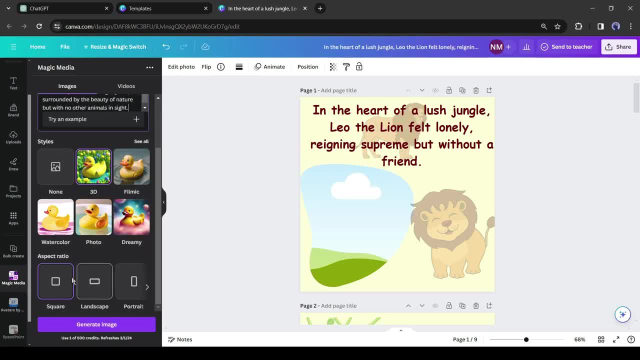 prompt, then paste it into the Canva prompt box. After that, you can change the aspect ratio. We will now want to create a portrait of the lion. We will create the image of the lion. After that, we will need to insert the color of the lion. We will want to create the color. 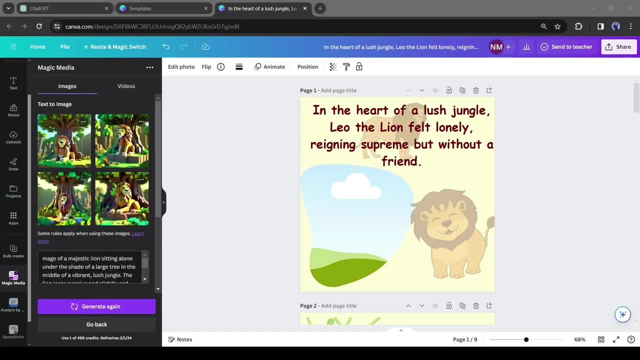 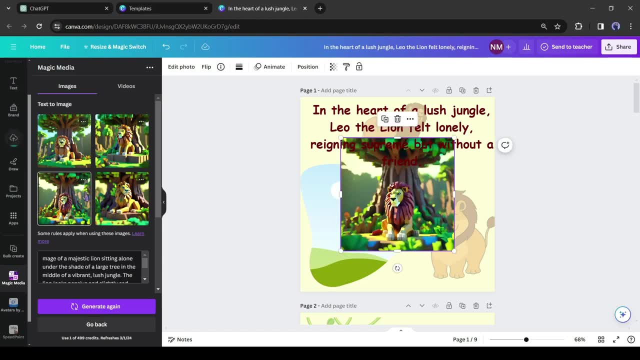 image button from here. It will take some time to generate the image And here it is. Canva Magic Media generates four images for us. Select one of them. You can see the art style is not perfect for us. Let's try with another style. This time I will go with the dream style. Okay, hit the. 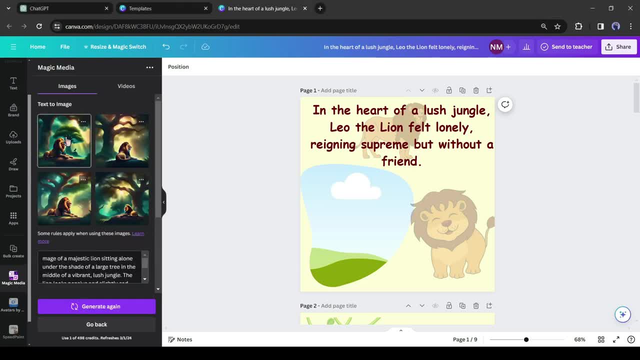 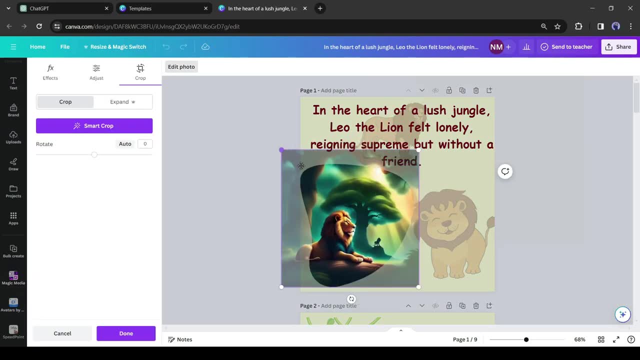 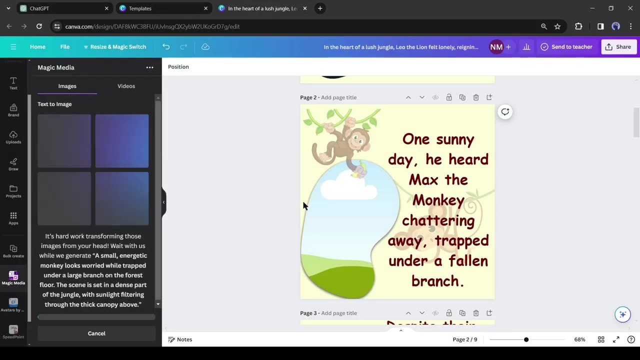 generate image button. And here it is. This time it generates better images. Simply drag and drop one image into the frame. You can adjust the size if needed. After completing the first page, go back to chat GPT again, copy the second scene and generate images with the same setting. 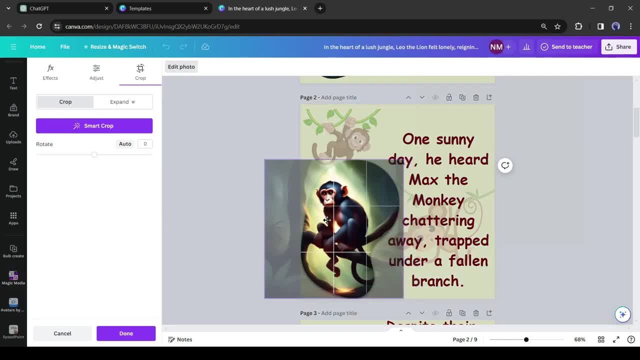 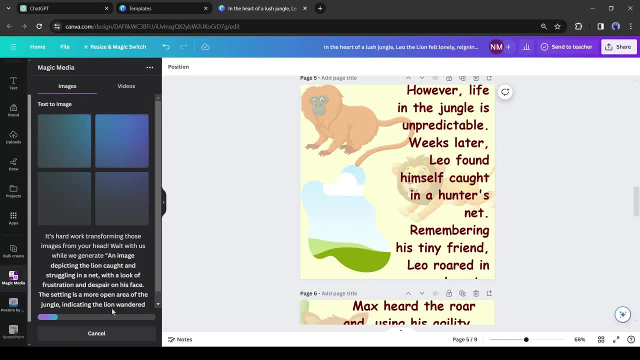 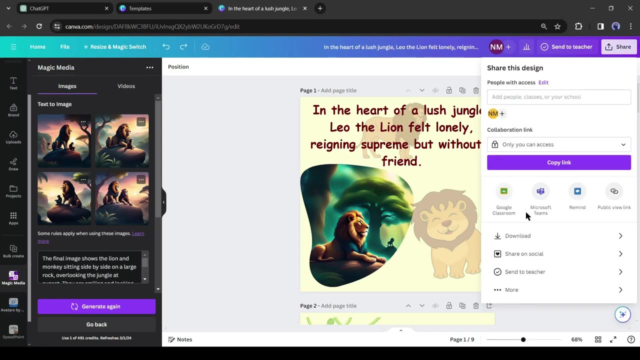 Insert the best image into the second page frame. In this way generates images for every scene and inserts them into the frame. We have successfully completed creating the story. To make the story a book flip, click the share button at the top, Then press the more button. Scroll down, then from the design section choose simple booklet.